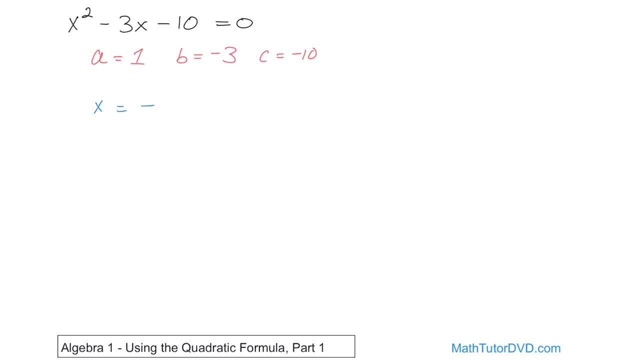 should memorize it, and it goes like this: X is equal to negative, b plus or minus, and I'm going to write b squared minus 4 times a times c, and the square root goes over all of these terms and then it's a giant fraction. 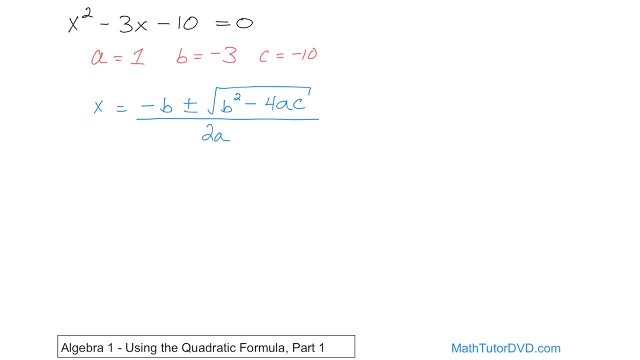 and on the bottom it's 2 times a. So that's really it. This is a plug-and-chug kind of formula. You stick a, b and c in here and then it just calculates the values of x and it works. 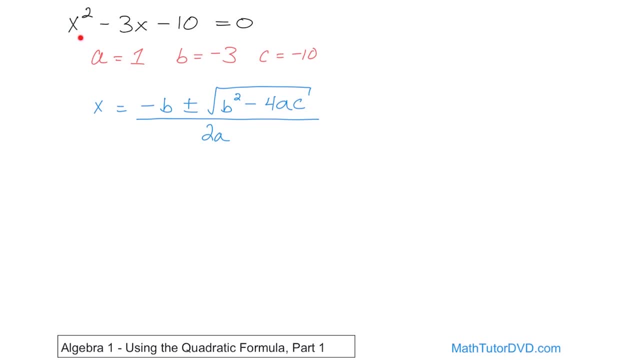 for any quadratic equation at all, anything of this form: x squared x and then a constant. you just stick the numbers in, So let's just crank through it. So the way you handle this is: you say x is equal to negative b. 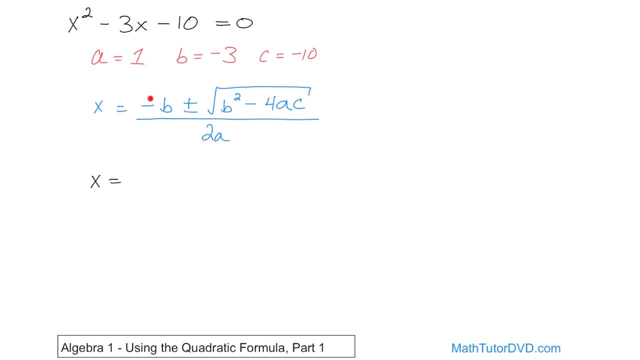 Now b is actually negative 3 in this case. so the formula says negative b. so don't do too many things at once, Don't outsmart yourself. The way you write it is negative 3.. So b is negative, and then b is negative 3.. 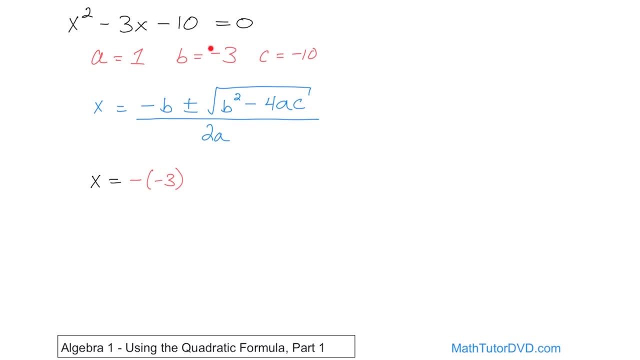 So this negative is just from the formula, The b is negative 3, so we're going to write that here. I'm not going to make this positive yet. I'll come in a later step. You don't want to do too many things at once. 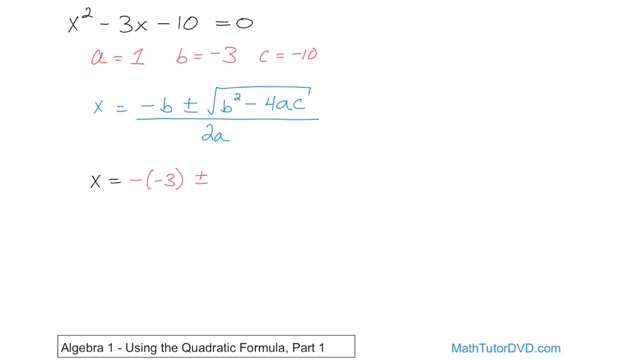 And then after that you want to write plus or minus, and then you have b squared minus 4ac. So b squared again. don't do the math yet, Write it as b. this is what b is squared minus 4 times a, which is 1.. 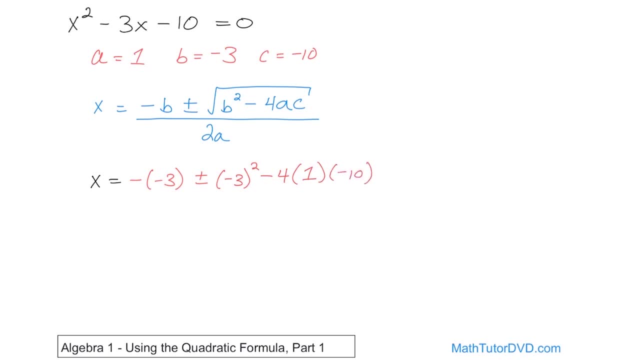 Times c, which is negative 10.. You write everything there. Don't forget that all of this is surrounded by a square root. and then you draw your big giant fraction bar and on the bottom it's 2 times a, which is 1.. 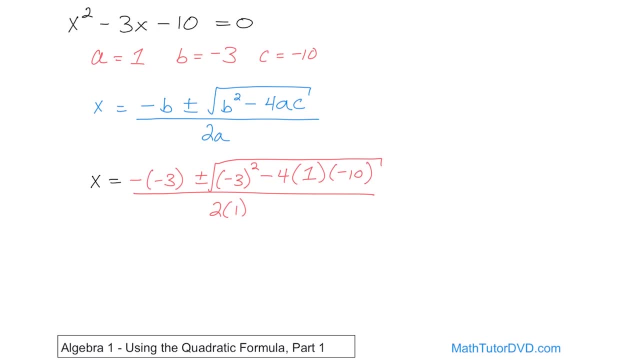 The reason you don't do too many things at once is because you will eventually make a sign error, You will forget something, and then you get the wrong answer for no reason. So you spend this step just writing down the numbers and then in the next step you continue. 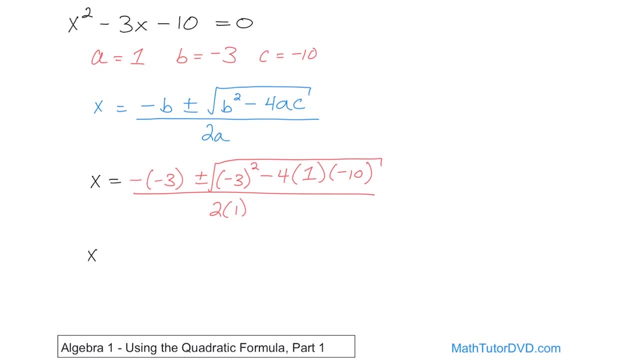 on with simplifying things. So here you have negative times. negative makes this a positive 3. The plus or minus always stays there, And then on the inside you're going to have negative 3 squared, which is positive, 9, minus. 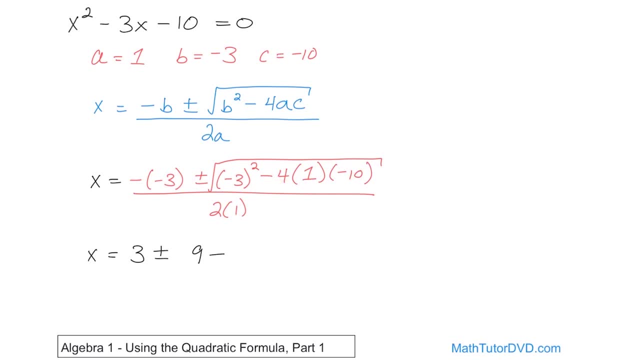 and then here you can do some math here: 4 times 1 is 4, and then times negative 10 gives you negative 40, right, Negative 40.. So this is negative 40,, right. But then you have this minus, so it's minus a negative 40, so that's basically a positive. 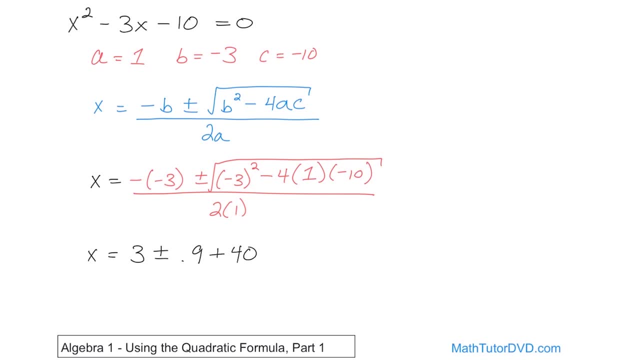 40. So here you have a positive 40 in here, And all this stuff is square root. Make sure you understand that. So here you have negative 40 from this. This makes it a positive 40. And then on the bottom it's 2 times 1, which is just 2.. 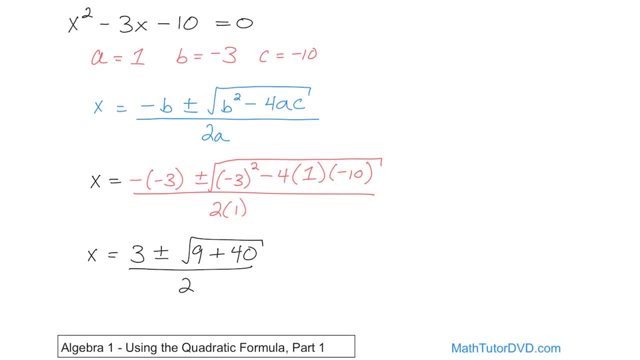 So you see how things start to clean up pretty fast. All right now what we're going to do is take this and we're going to continue writing down or simplifying here. So x is going to be equal to 3 plus or minus the square root of 9 plus 40,, which is 49,. 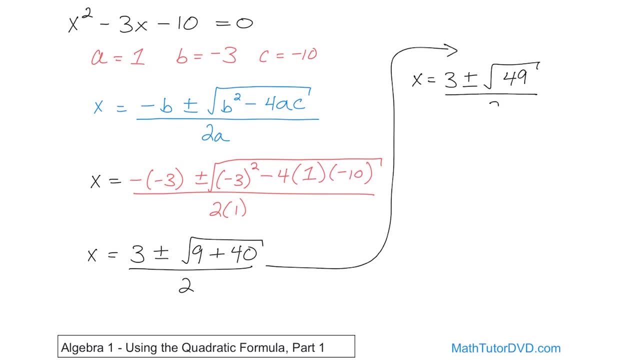 which is nice, because 49 is a perfect square, so we'll be able to simplify that in the next step. So then we know that x is 3 plus or minus. what is the square root of 49?? You should know that. 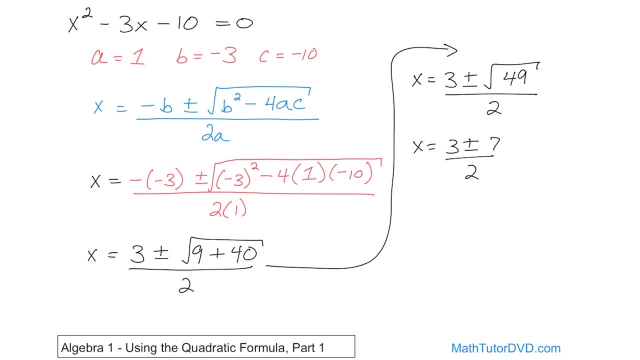 7 times 7 is 49 over 2.. Now, really, you almost could circle the answer here, because this is really the answer, But this plus or minus really means that there's two answers here and you want to drill it down as far as you can. 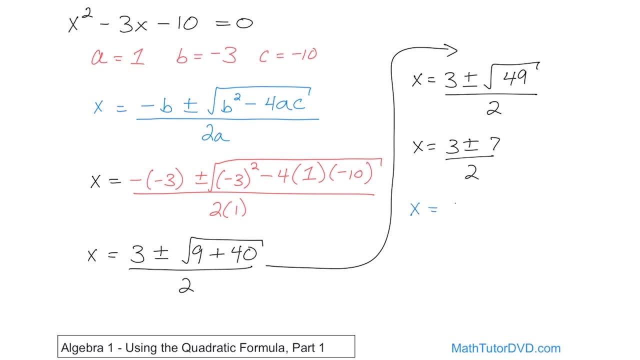 So we want to write down both answers. So the first is on the top. if the plus is selected, it's 3 plus 7 over 2,, which is 10 over 2, which is 5.. So the first answer is that x is equal to 5, just like this. 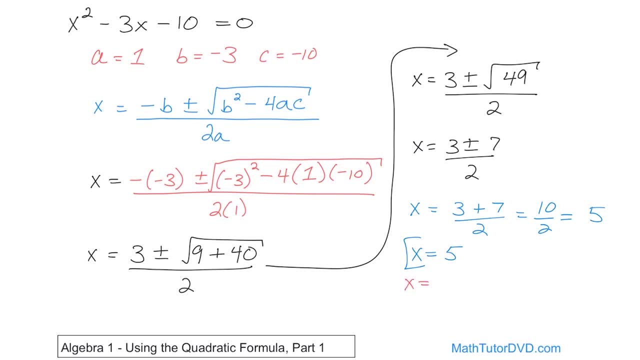 And the second answer. I'll do that one in red is: x is equal to, if you select the minus sign, 3 minus 7 over 2.. Now, on the top: 3 minus 7 is negative 4.. What's negative? 4 divided by 2 is negative 2.. 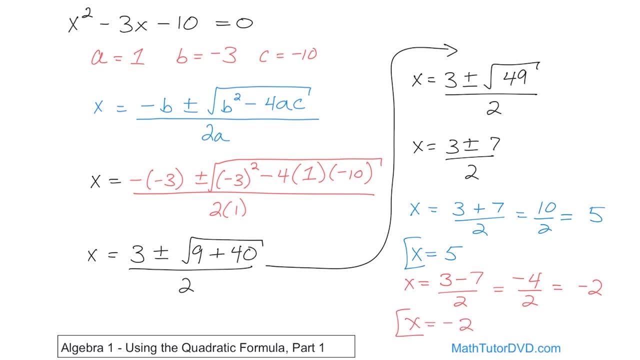 So it's x is equal to negative 2. And that's the final answer, right there. So what you see at the end of the day, when you finish all this thing, is that any quadratic formula, any quadratic equation, you can use this quadratic formula, which you should. 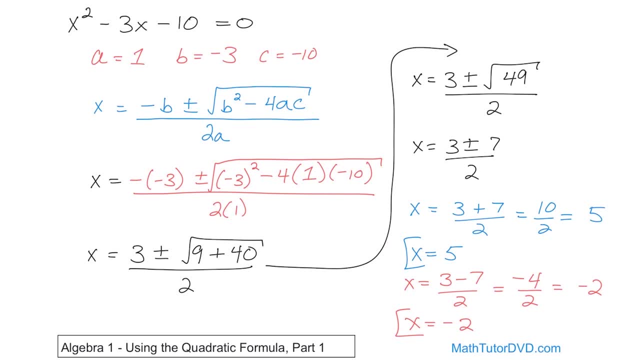 memorize And when you crank through it you're always going to get two numbers. Two answers are always going to come out, because you have a plus minus in the quadratic formula. This 5,, if you stick it in here, will satisfy the equation. 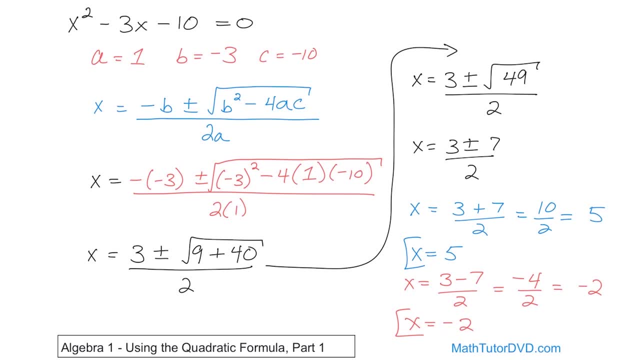 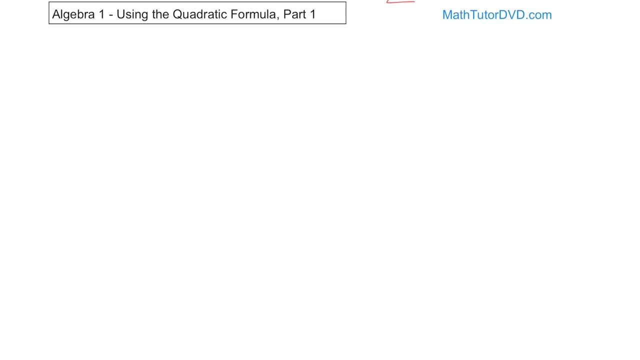 This negative 2, if you stick it in here, will also satisfy that equation. So now that we've got the basic idea out of the way with the first problem, now we're going to crank through the remaining problems a little bit faster. 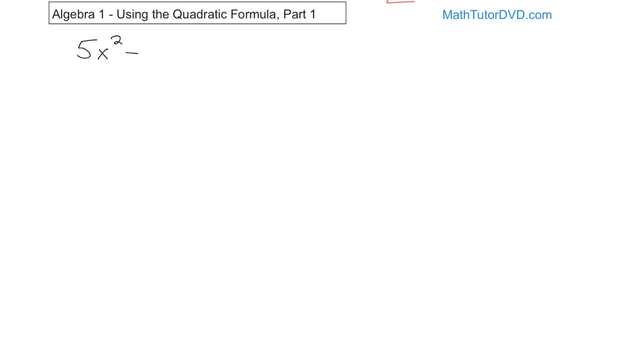 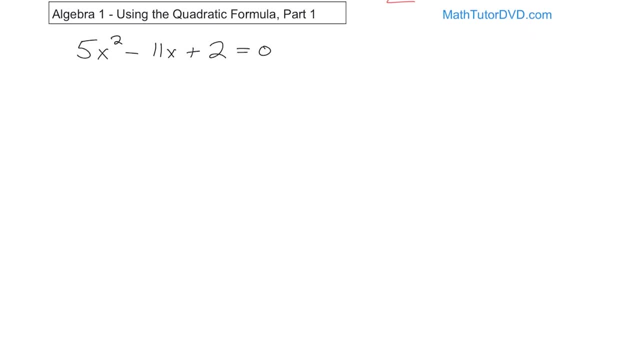 7x squared, 7x squared, 9x squared, 9x squared. I actually want to probably Ahí là t TSB, but this is not going to be as rhinic than I think that I would expect it to be today. 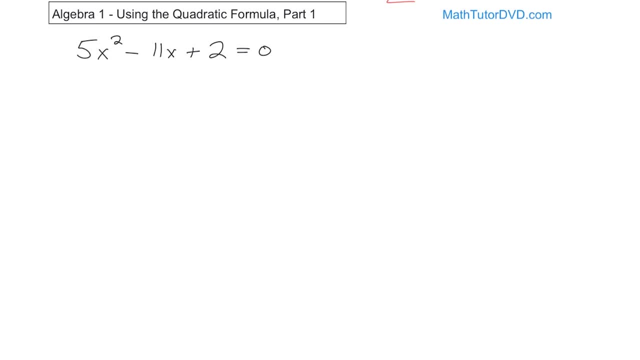 So we're going to go ahead and get this all out of the way here. That's why I don't want to go over it too much. 11, and c is equal to 2,- just the three numbers that are in this problem. and then we always. 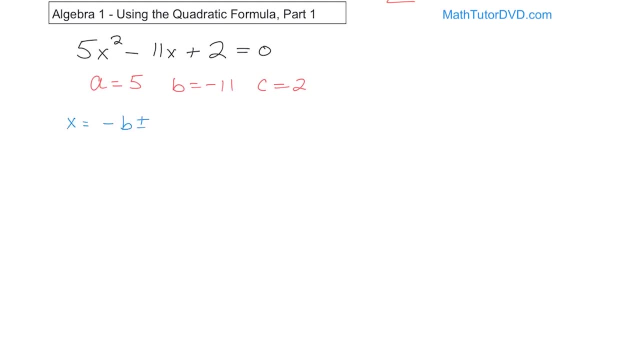 write our quadratic formula, even if you've written it a million times: plus or minus b squared minus 4 times a times c, square root goes over that over 2a, and then we just start plugging things in, so we'll switch to black for that. so x is equal to negative. 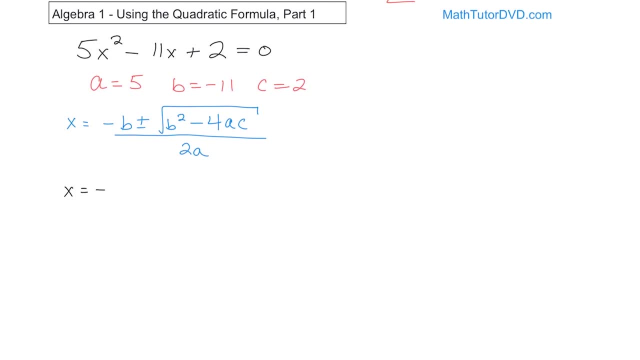 b. so the negative sign comes here. but b itself is actually negative. so you put it in parentheses: negative 11, plus or minus. then you have b squared, which is negative, 11 squared minus 4 times a. but a is 5, times c is 2, square root goes around all of these. 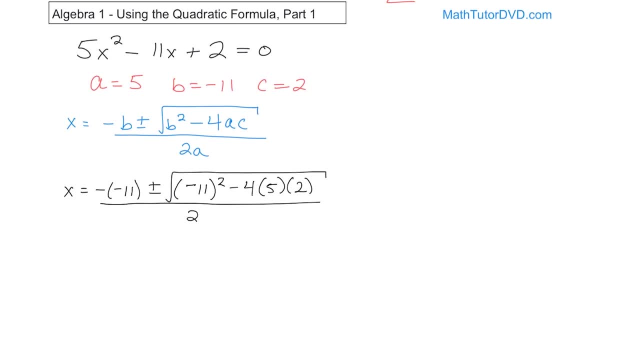 numbers. all of this floats over a fraction bar 2 times a, but a is 5, so again your first step: you put those numbers in. you don't try to do any multiplication or anything, because you want to keep everything as clean as you can to trace your work, if you make. 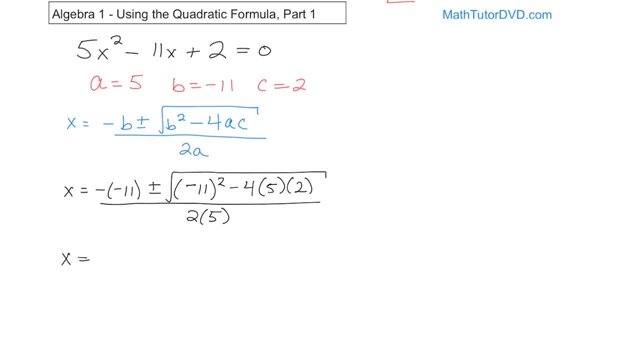 a mistake somewhere. All right, so now we go down here for the first step: negative times. negative 11 gives you positive 11, plus or minus, and inside of here negative 11 squared is going to be positive 121 minus. and here's where you can do a little bit. 4 times 5 is 20, times 2. 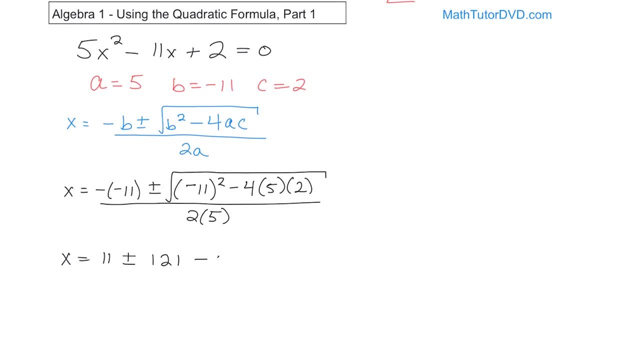 is 40,. the minus sign is still there, so it's minus 40 or negative 40, the square root wraps around there and on the bottom: 2 times 5 is 10,. all right, 2 times 5 is 10..